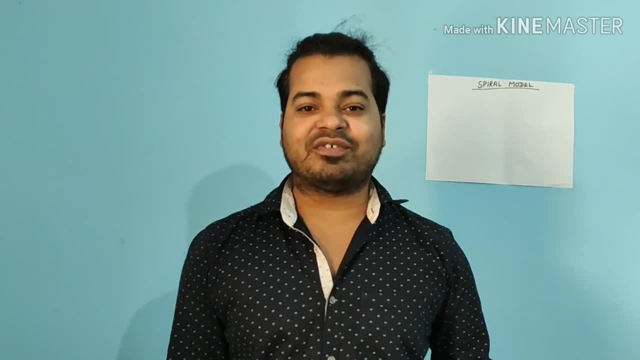 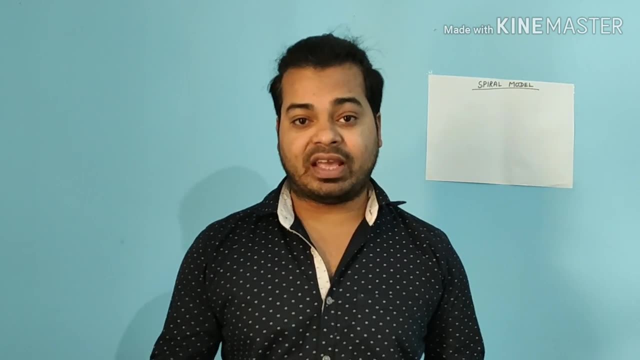 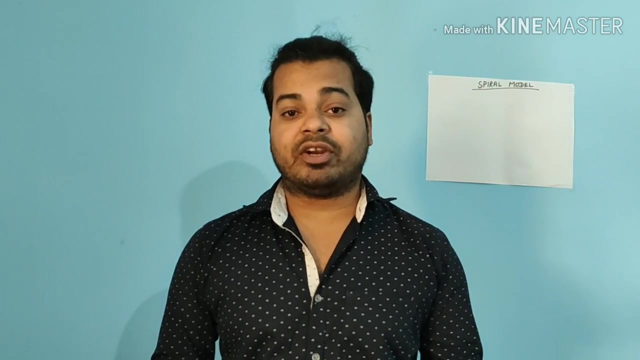 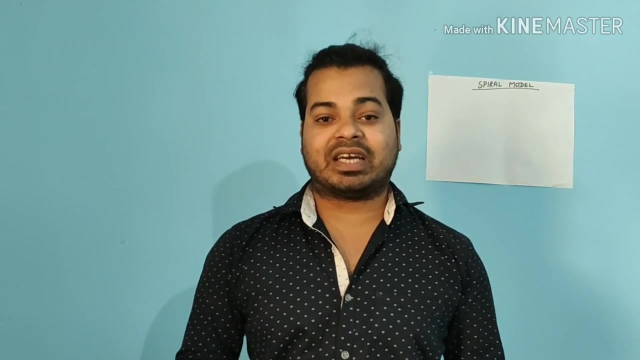 Hi guys, I welcome you all to another video of software testing by MKT. So in this video I'm going to talk about what do you mean by spiral model as a software development life cycle. Before we proceed with this video, make sure that you have watched my waterfall model video and also software development life cycle video. If you have not, you won't understand this, So I will request you guys to watch that first and come to this video. Let's get started. 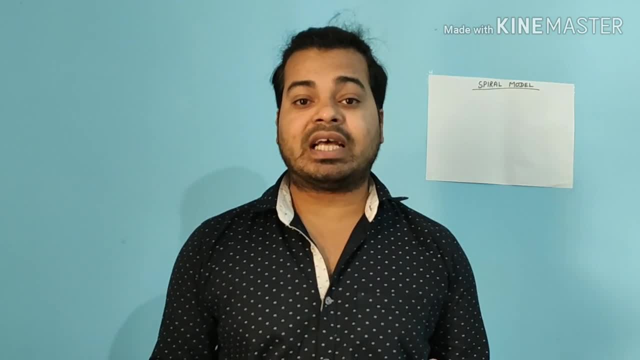 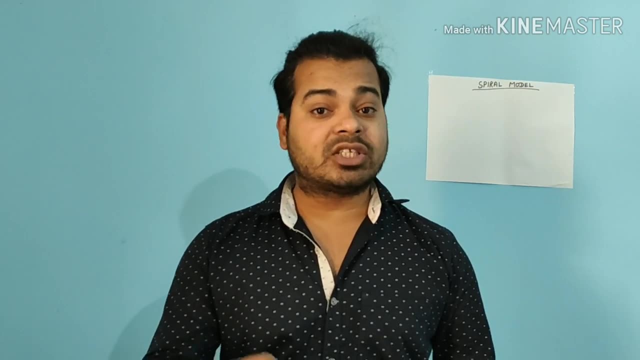 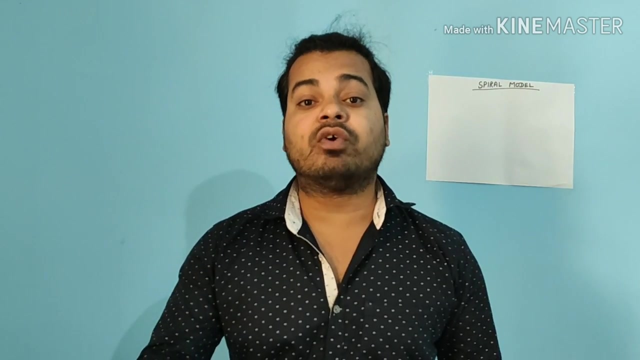 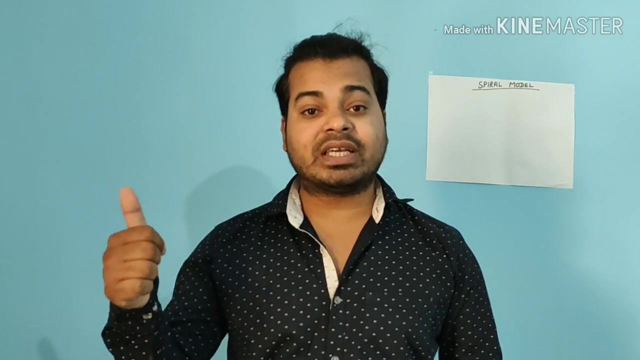 Okay, so spiral model as a software development life cycle. It is a step by step procedure or a standard procedure to develop any software And in order to avoid the drawbacks of waterfall model, we go for spiral model. Understanding guys? So if you remember, I had told you guys that what in waterfall model? once after the feasibility study is done, you cannot go back to the spiral model. 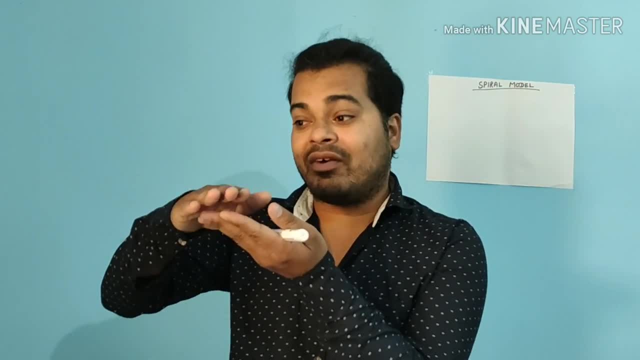 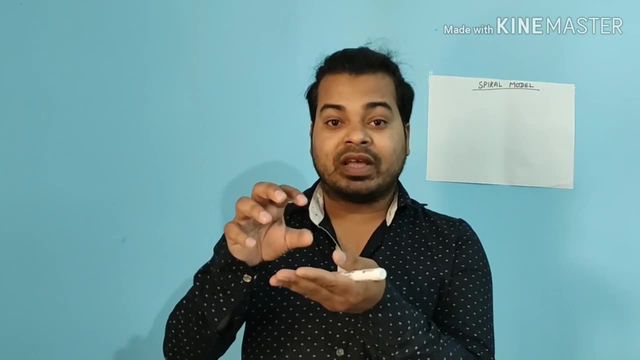 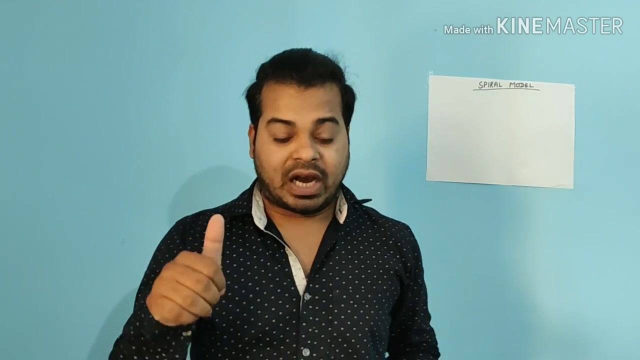 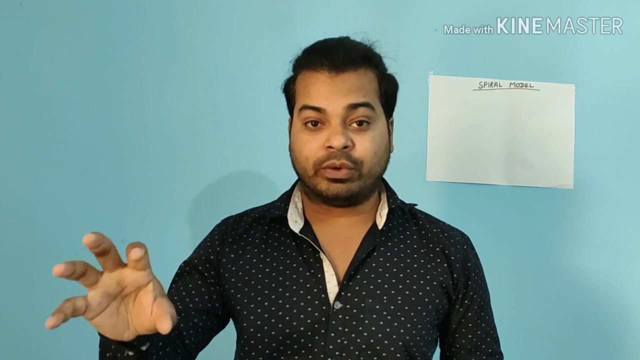 You cannot go back and change the requirement. Requirements will be freeze. You have to only go in this direction. I hope you guys remember very well. So in spiral model, in order to avoid that drawback, we go for spiral model. I hope it is very understanding. Other than that, we follow spiral model whenever there is a dependency between the modules. Listen to me very carefully, guys. Now I'm going to tell you what is a spiral model. 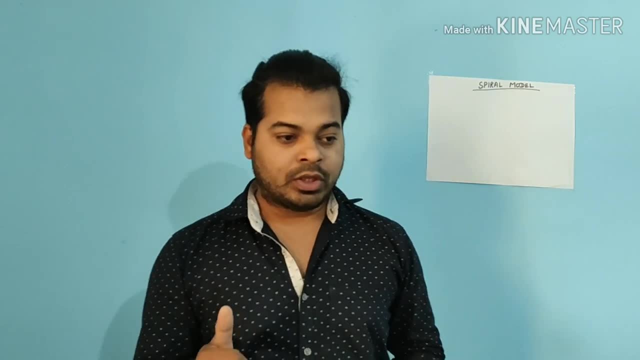 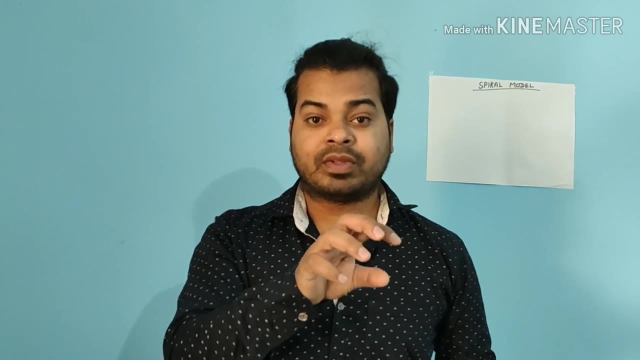 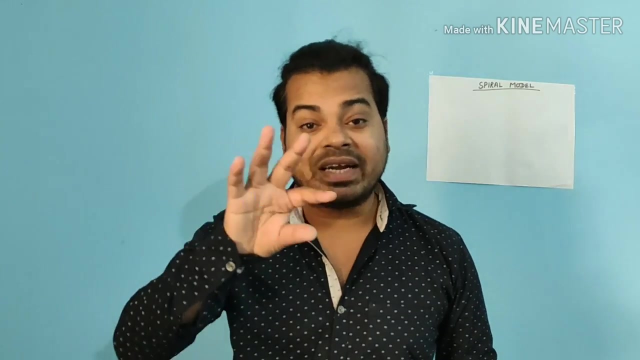 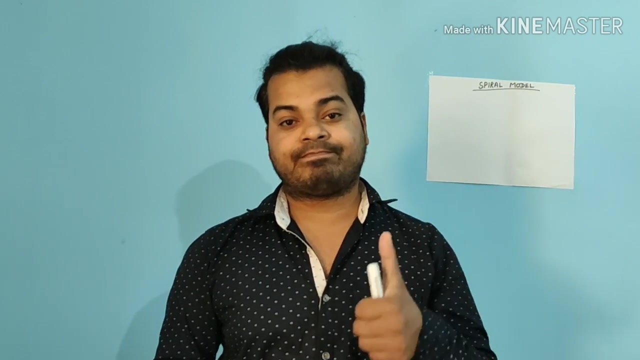 What do you mean by dependency and what do you mean by modules? So what do you mean by dependency? Dependency means when one module is dependent on another. Now, what do you mean by modules? Module is any feature. When one feature is dependent on any other feature, that is called as dependency. So whenever there is a dependency between the two modules, we go for spiral model. I will show you the pictorial diagram how it looks like. 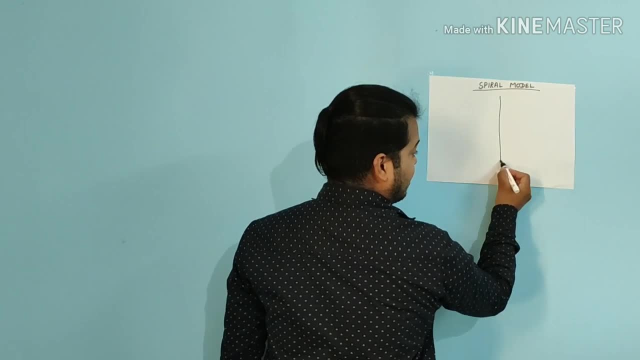 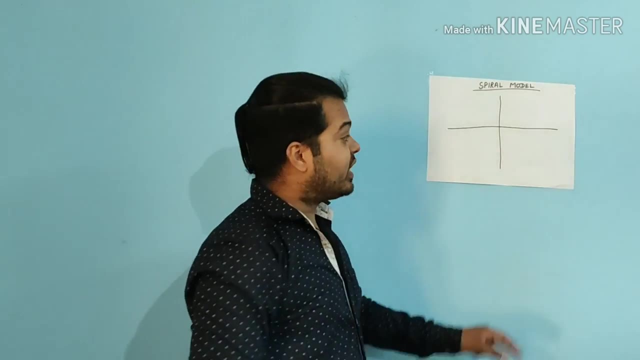 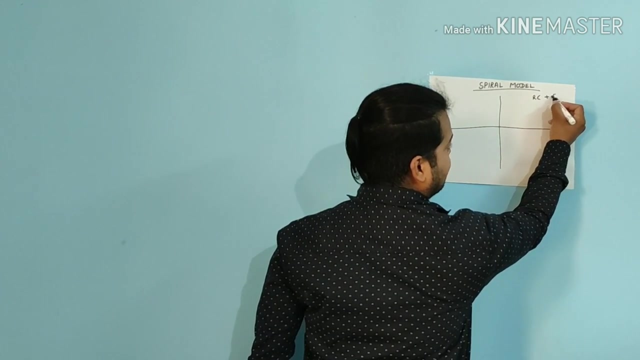 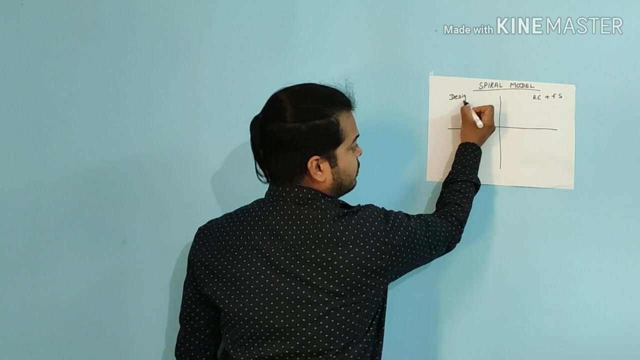 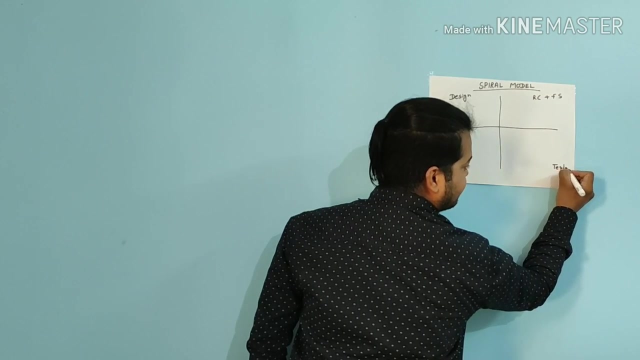 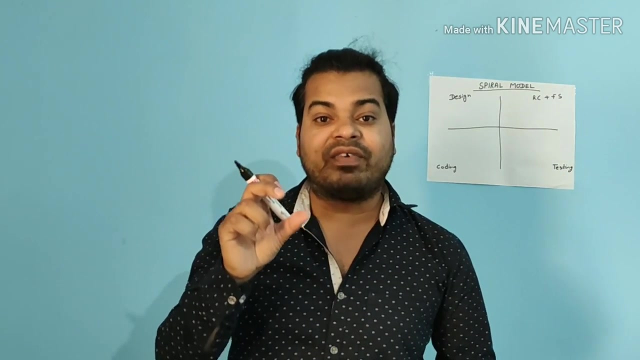 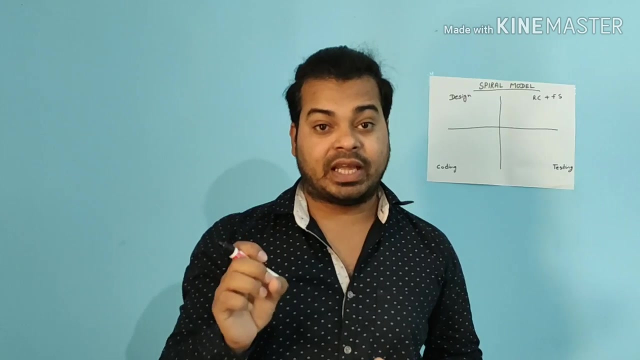 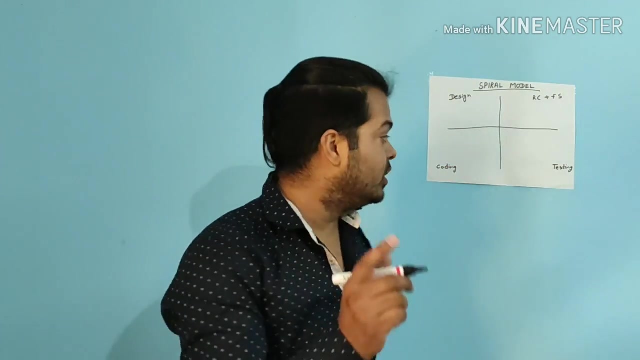 So in spiral model we mainly have four sections. In the first section we do requirement collection and feasibility study, Requirement collection plus feasibility study. In the second phase we do design And then here we do coding. As I have said to you, we follow spiral model. whenever there is a dependency between the modules we go for spiral model. I will show you how spiral model looks like. So suppose requirement has come for a module, particular module, let's say one module. So this is my first module. 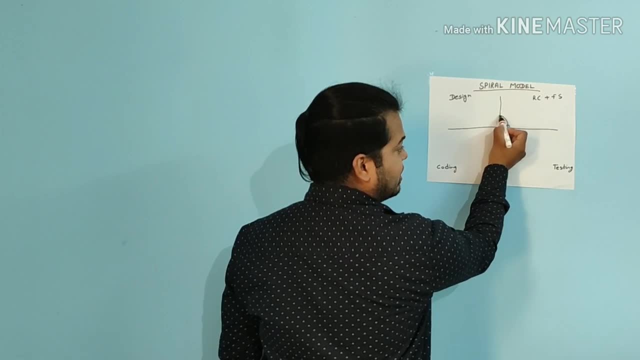 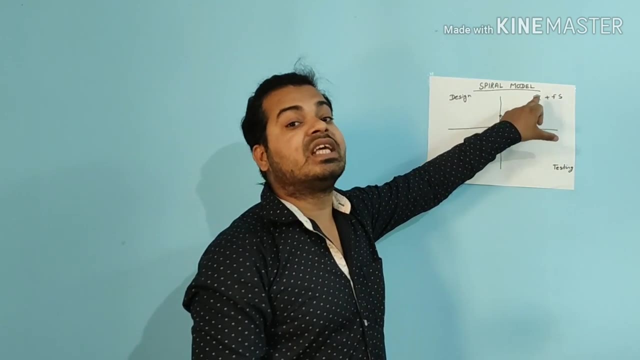 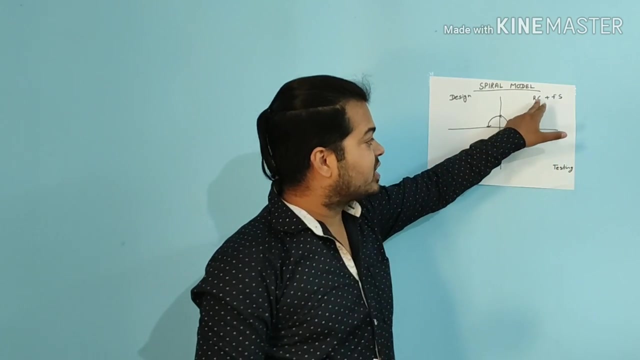 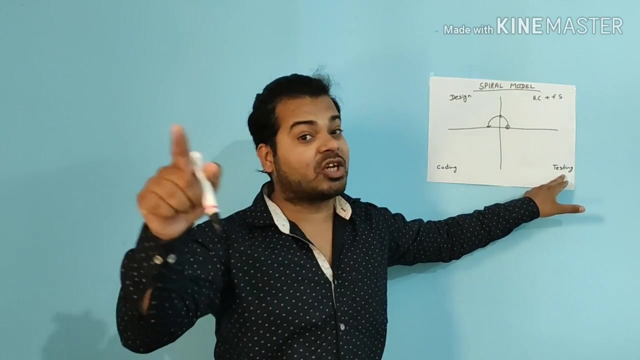 Requirement is done And corresponding feasibility study is done. Once after my requirement collection and feasibility study is done, I will go for design. You guys will not understand what is requirement, collection, feasibility study, design, coding testing unless you guys have watched my software development life cycle video. Make sure that you have watched and come here. 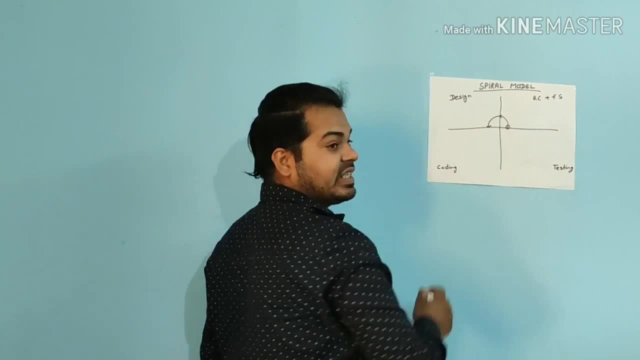 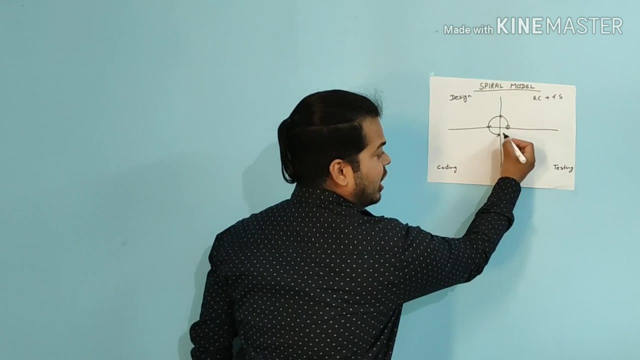 So suppose for module first, requirement, collection and feasibility, Yes, Yes, Yes, Very good. So for module first, requirement, collection and feasibility study is done, then design is done, Then for that coding is done. Now we have to do testing for this particular module, that is module number one. 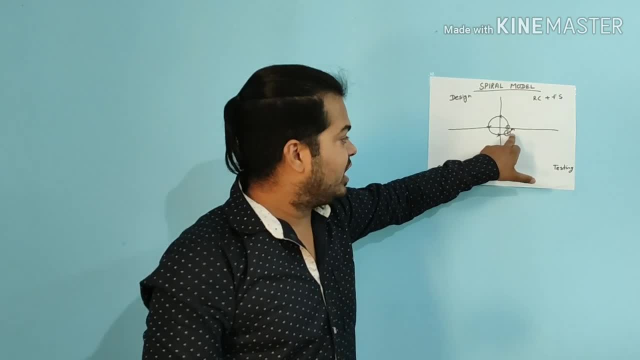 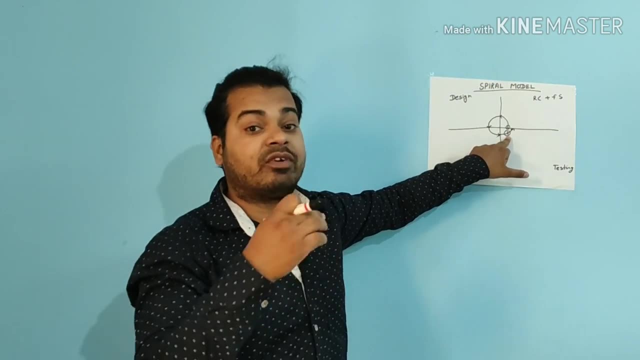 Yes, Yes, Yes, Yes. While testing it, if we get any defect, we have to communicate with the developer. They have to give the new software. We have to test it, We have to test it carefully And if no defects are there, we are finally going to release this software to the developer. 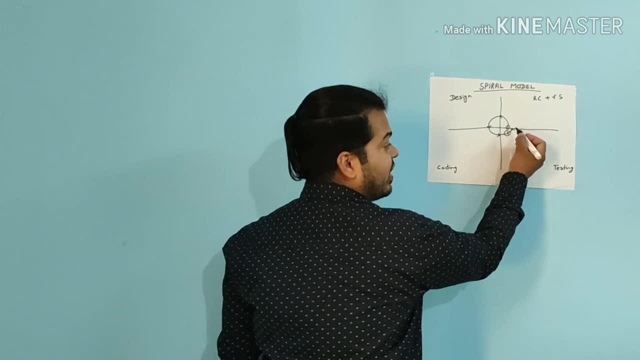 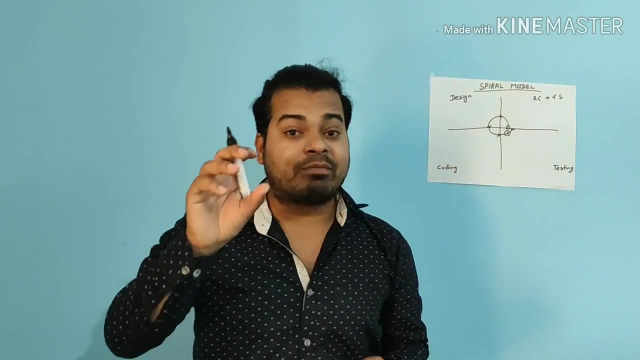 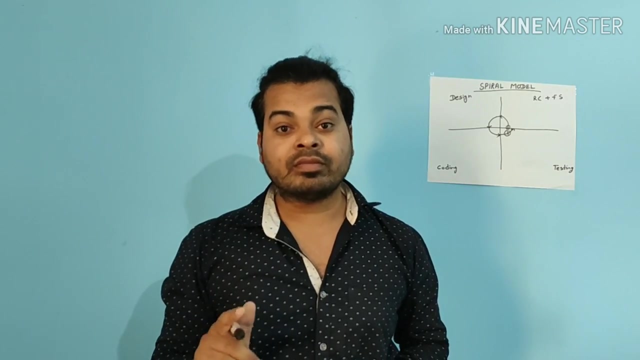 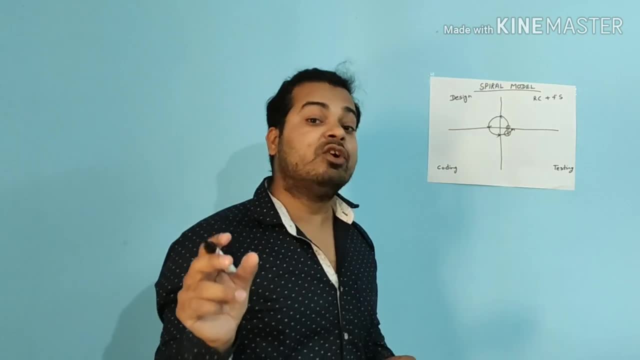 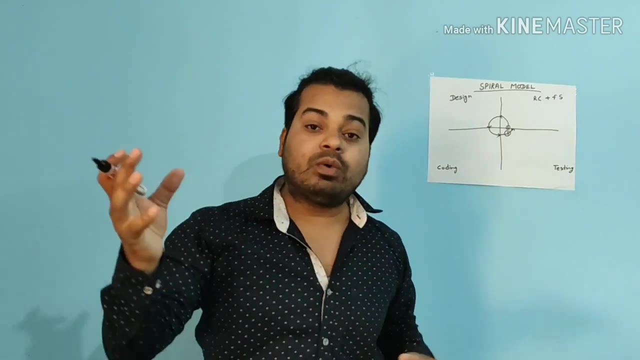 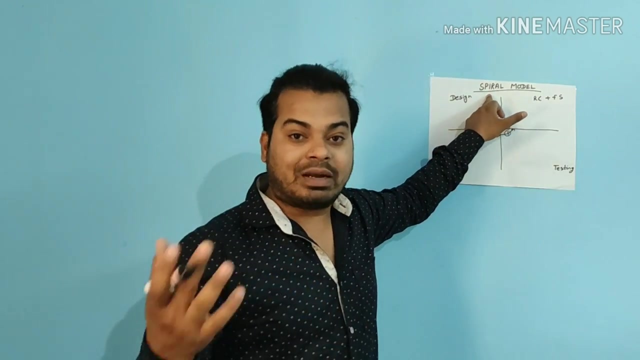 more point. Now, when new module is coming here, what happens? Since we have worked on module A, right, we can release it to the customer now. Now requirement can come for the module number two. Here we test it like that. So in SpiralModels we follow that. 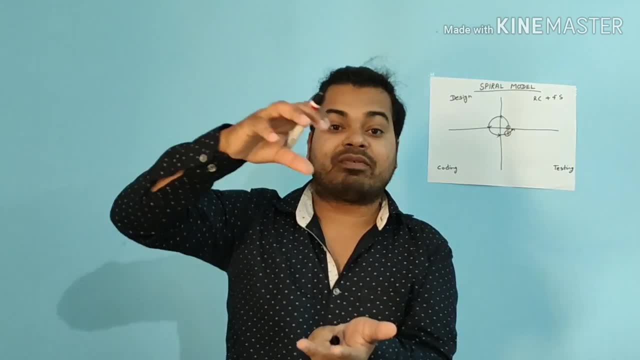 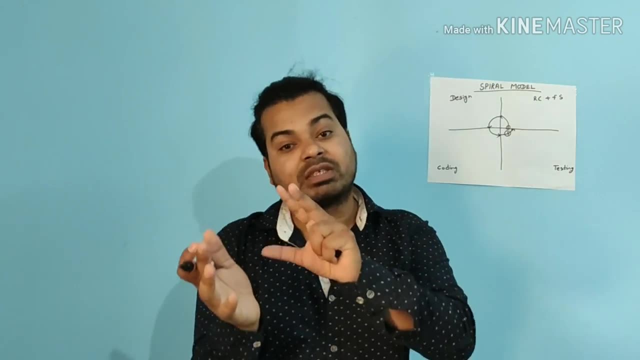 method: We take one module, we test it, we release it to the customer. when that module is stable, Then only we take the second module. We test it and then perform the integration between the first module and second module, test everything, then we release it to the. 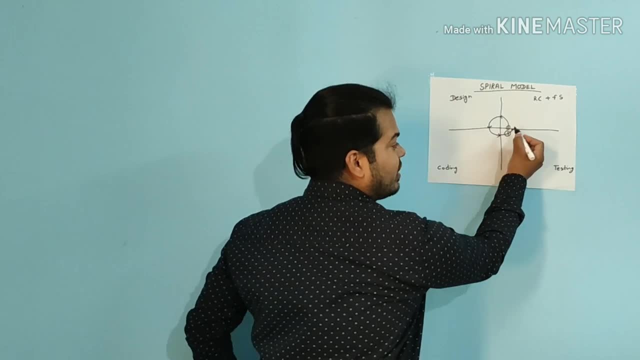 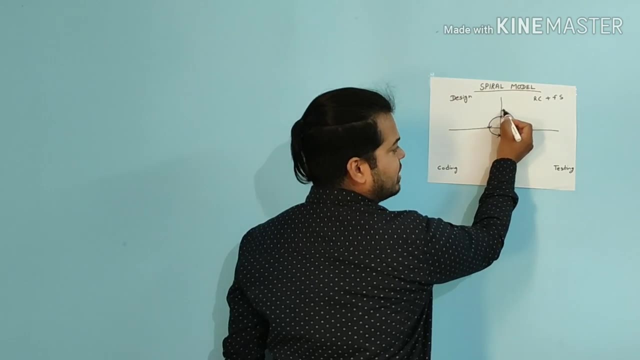 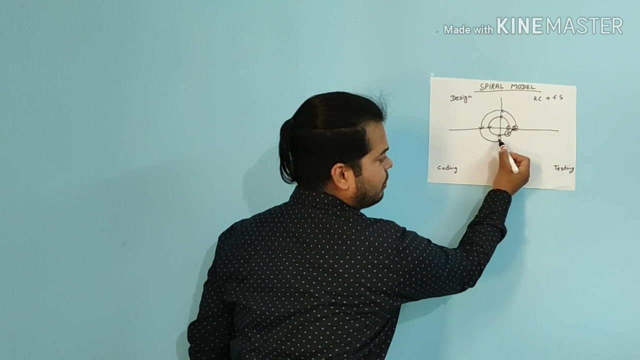 customer. Now, customer will give requirement for module number second. Now requirement collection and feasibility Study has to be done. Once that is done, then architect will do design, Developers will do coding Test engineers will do testing. Now, if you remember, I am testing my new. 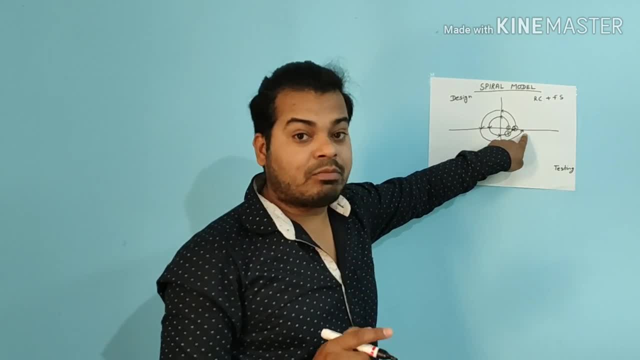 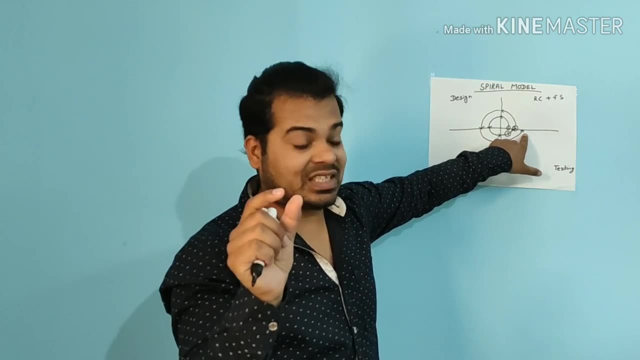 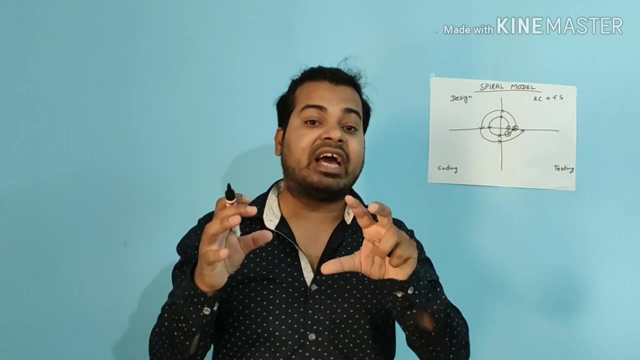 module second. Now in this particular module I have module number second and module number first. How I am gonna test this particular phase In this part. whenever I am testing a new module in which I have one more module previously, that is module number first. How I am gonna. 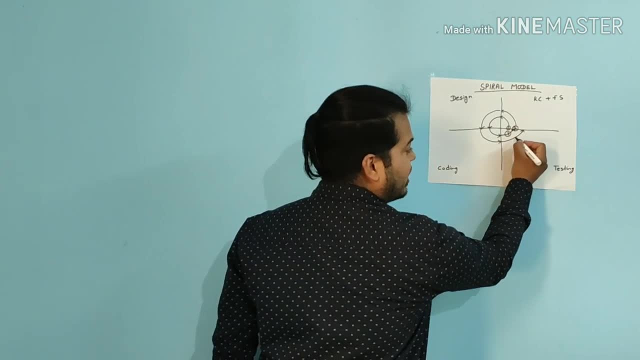 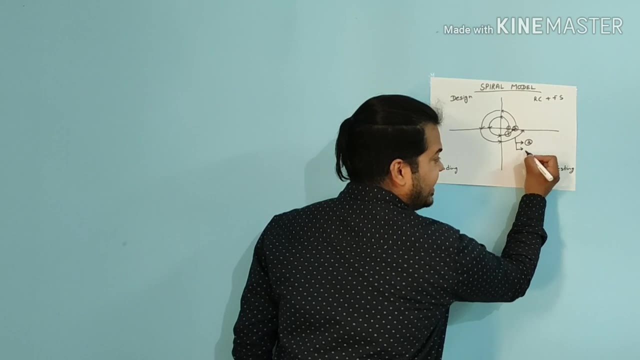 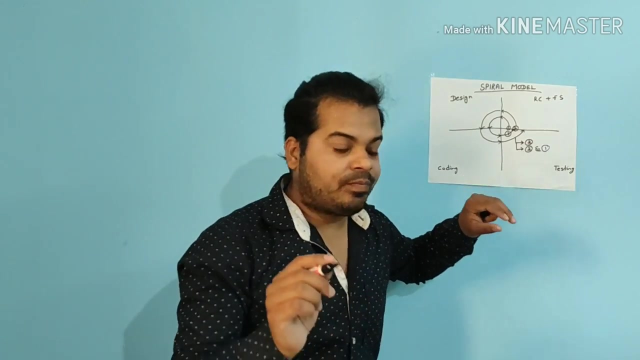 perform the testing here. So how I am gonna test this, I am gonna test the module number second first. Then I am gonna perform the integration between the second module and first module. So I will first perform the testing of module second. That is my newly. 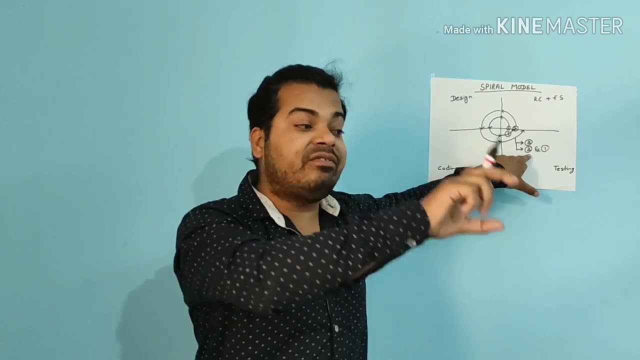 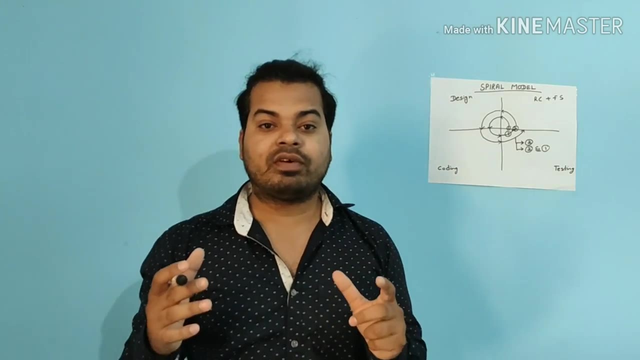 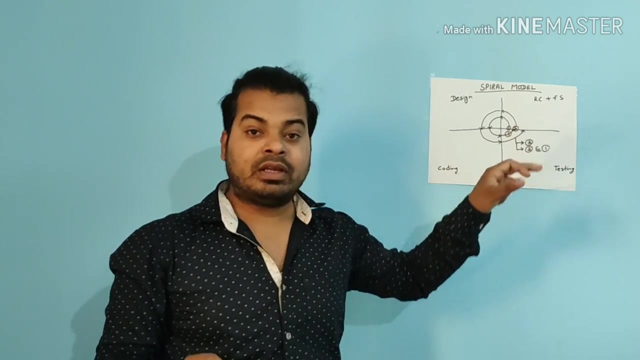 module, Then I will perform whether the newly module and previously module Integration between them means. let's take an example of Gmail. If you are composing a mail, that composing a mail is a one module. That is module number first. Now module number second. let's say 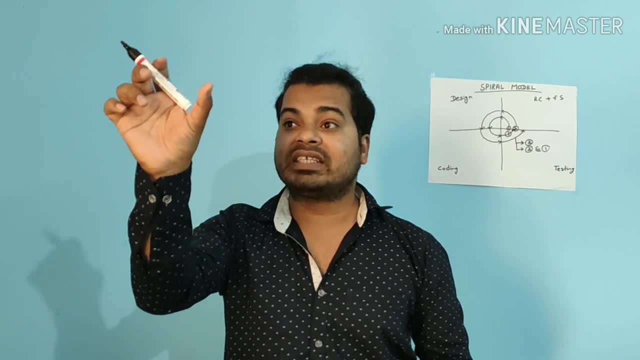 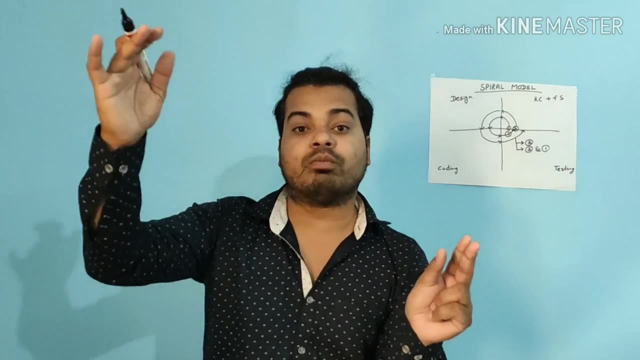 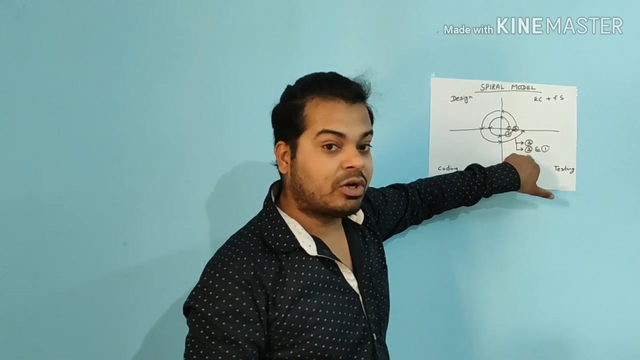 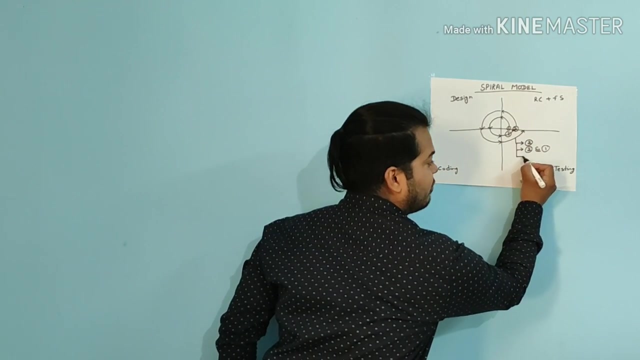 you have sent items Until, and unless you send a mail, it can't come to the sent items. That is called as integration between the two modules. Are you guys getting me Great? So I will perform the integration between the second module and first module And finally I am gonna test the module number first To make 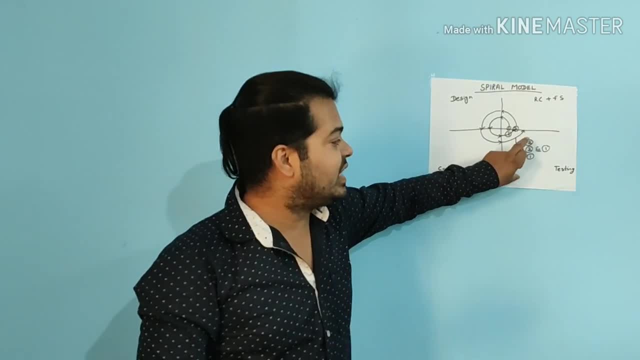 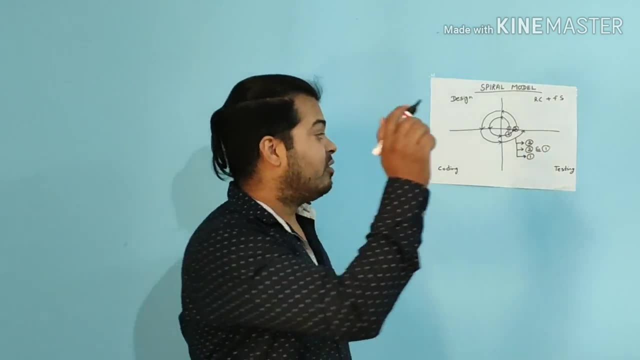 sure that just because by adding second module, does it affecting the module first? For that particular reason, I will test first newly added module, Then my second module. I will test the module number first, Then I will perform the integration between the two modules. 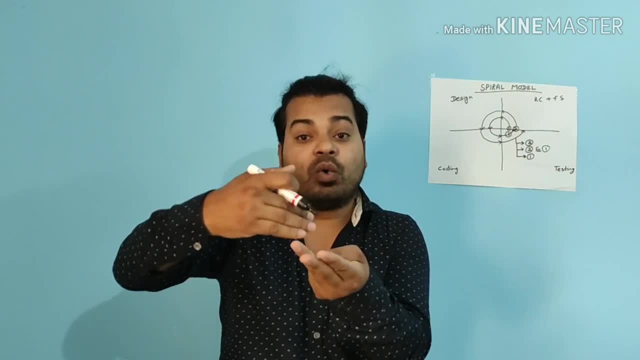 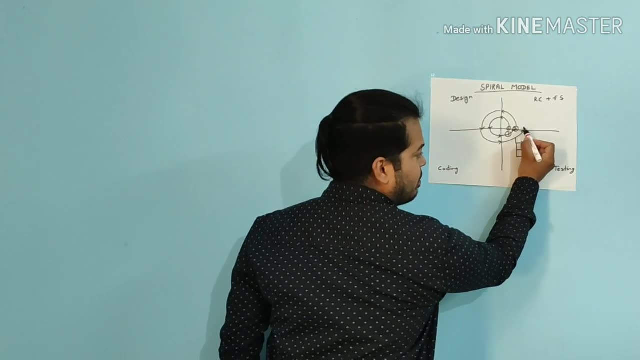 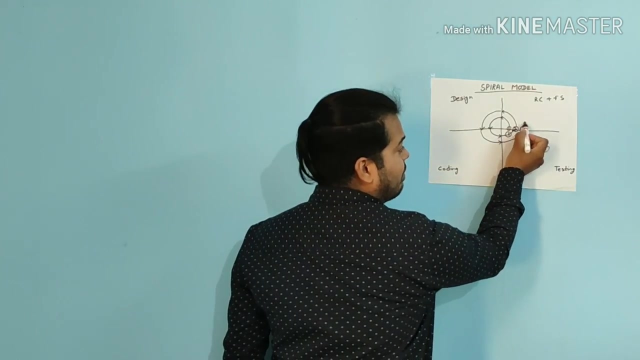 Finally, newly added module plus it's integration with the old modules and then finally the old modules. Guys getting me Now suppose the requirement has come for the module number. third, Newly module has come: Requirement collection, feasibility study will be done. Architect will do design developers. 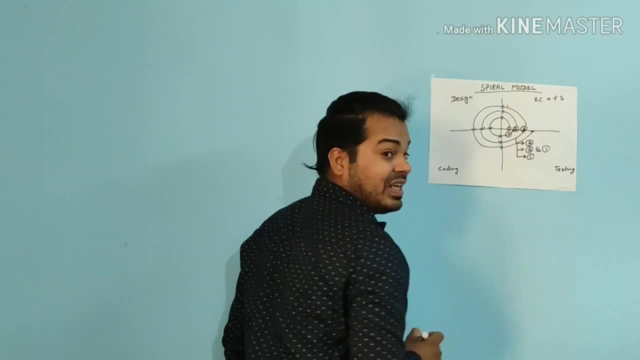 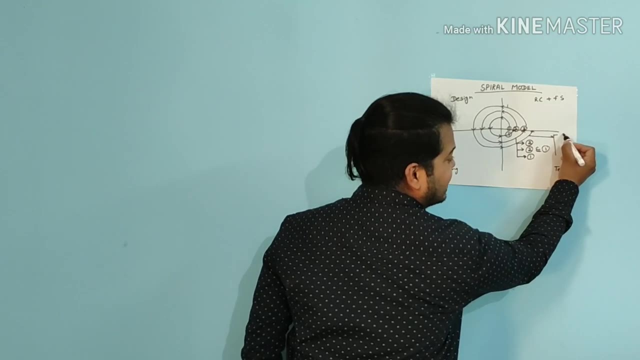 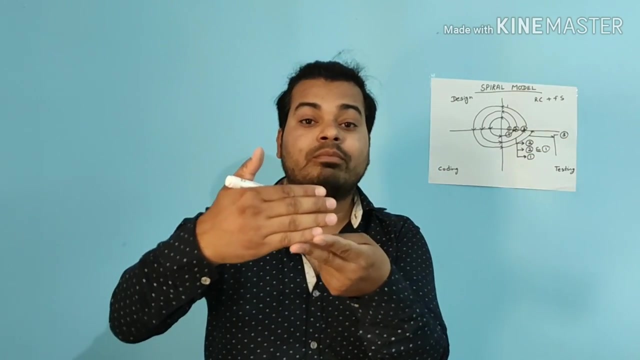 will do coding. Finally, test engineers how they will perform testing. here We make a. So, since it is a new module, what test engineers will do? They will test the newly added module first, that is, module number 3. And they are going to perform the integration between the new module and the old module. 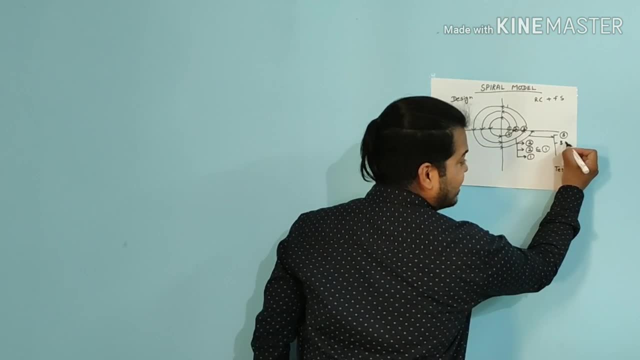 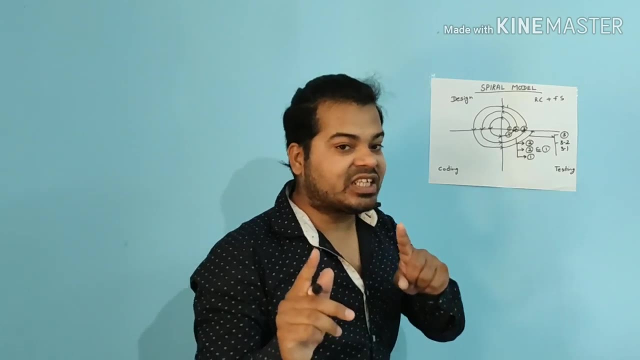 So they are going to perform the integration between 3.2 and 3.1.. That means they will perform the integration testing between module 3 and module 2.. They will perform the integration testing between module number 3 and module number 1.. 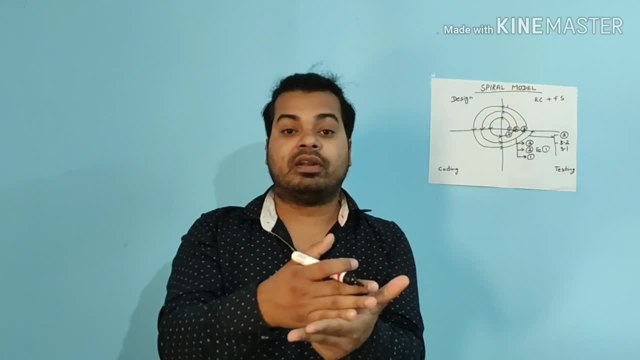 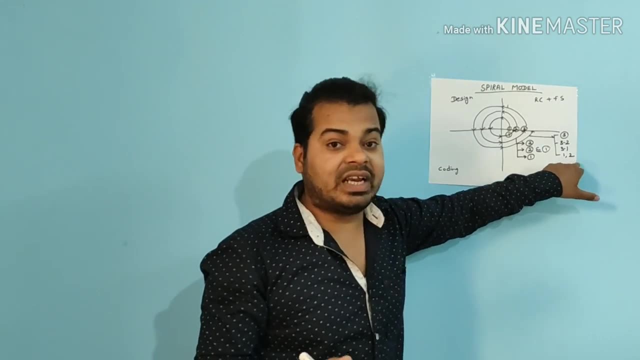 And finally, they are going to test the old module. To make sure that they are going to test the old module, that is first and second. Now, why are we testing module first and second? The reason is just because by adding module number 3, is it affecting my old modules. 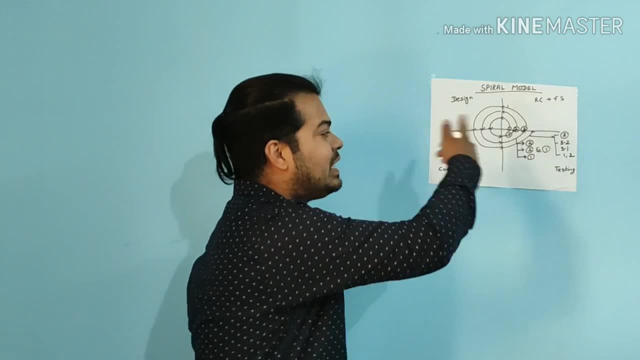 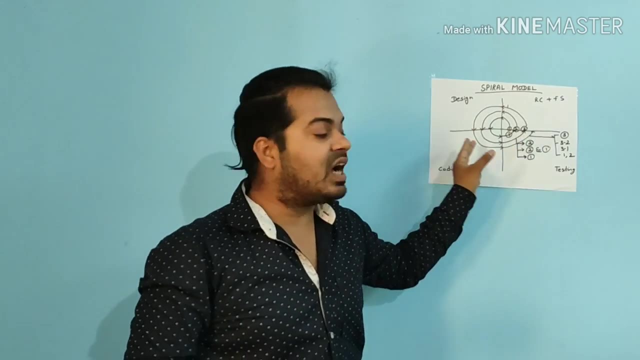 To make sure that I will perform testing like this: It will keep on recording, it will keep on repeating guys, It will keep on repeating Modules, keep on adding. We perform the same cycle again and again. I hope it is very clearly. 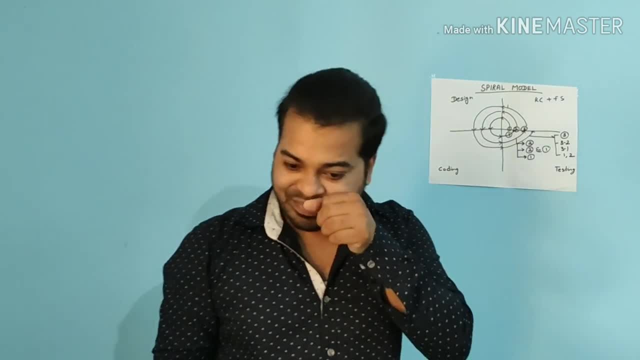 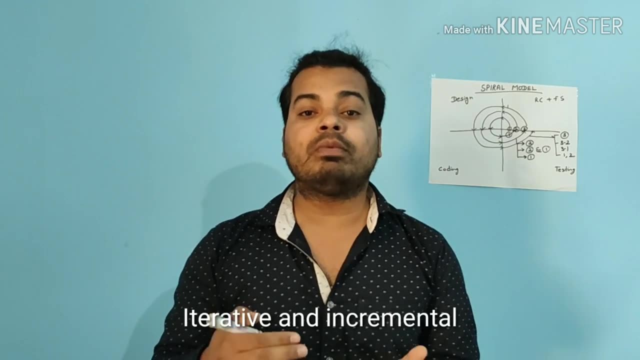 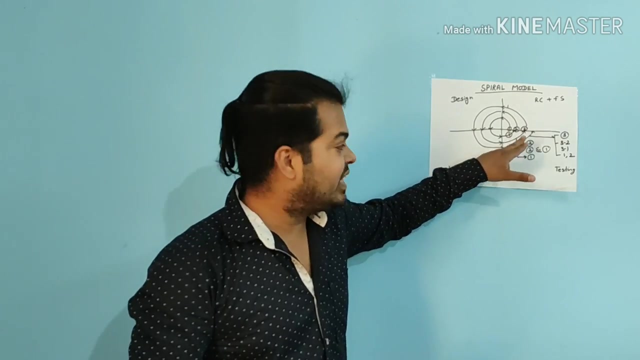 I have explained in a very easy language, Guys. spiral model is also called as iterative model and incremental model. Now what do you mean by incremental model? Incremental model, we say, because here modules are keep on repeating, Modules are keep on increasing. Module number first and second and third and fourth, fifth, sixth. That is why we call as incremental model. Now the question arises why it is called as iterative model. The reason it is called as iterative model is because we perform the same cycle. we perform. 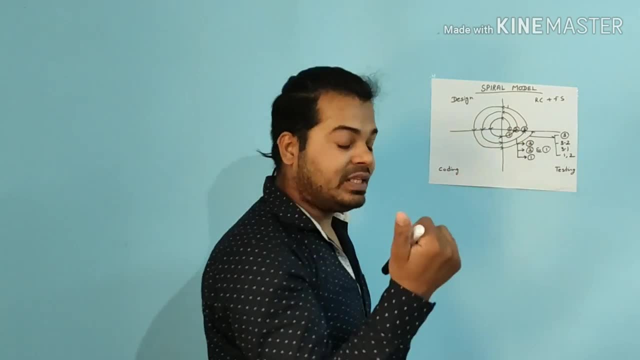 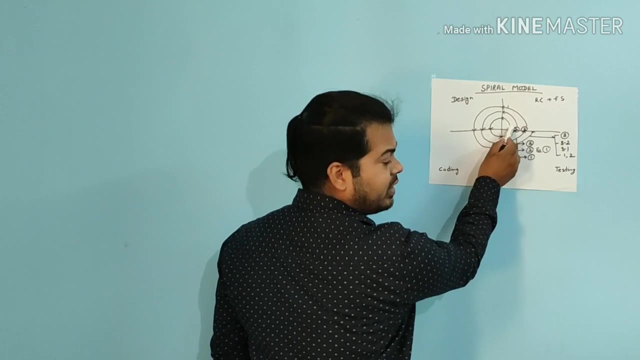 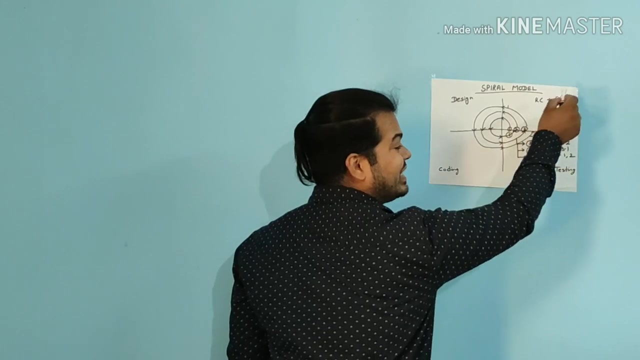 the same process in each cycle. That means this is my one cycle, guys. Starting from here, then releasing to the software, Starting from here, Requirement collection, feasibility study, design, coding, testing and finally releasing to the customer. This is my one cycle. 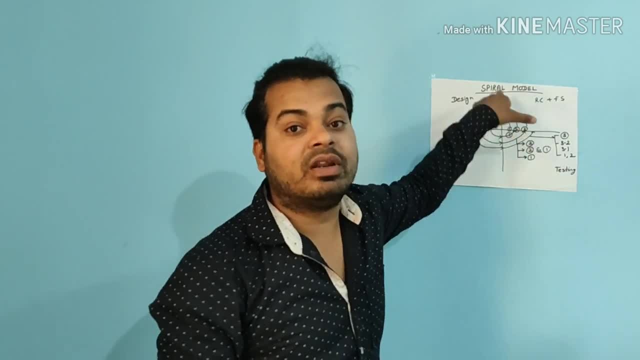 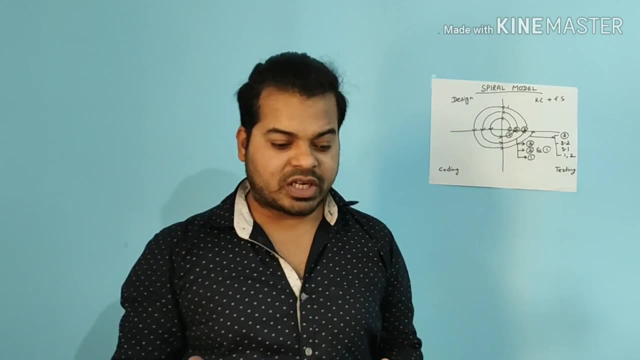 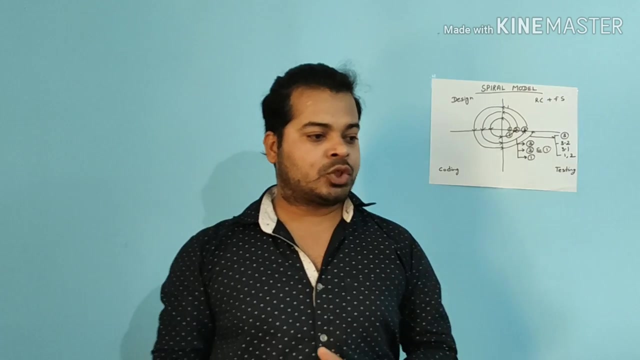 Same process I will be repeating for each and every module. That is the reason it is called as iterative model. Great. Now the question arises: what are the advantages of choosing spiral model in software development life cycle? So the best example of spiral model is: 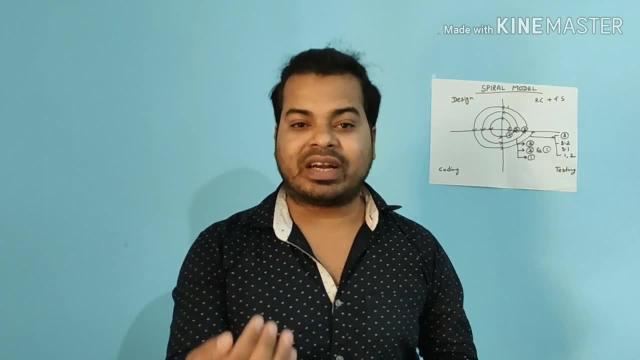 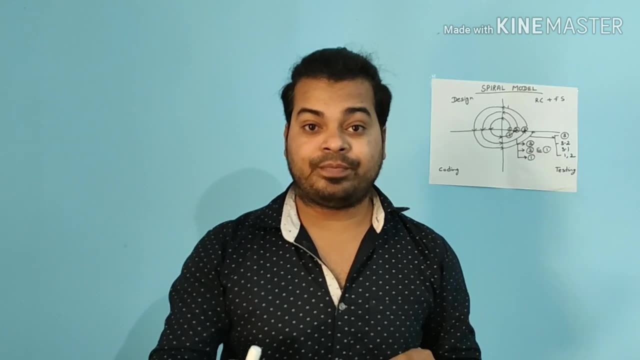 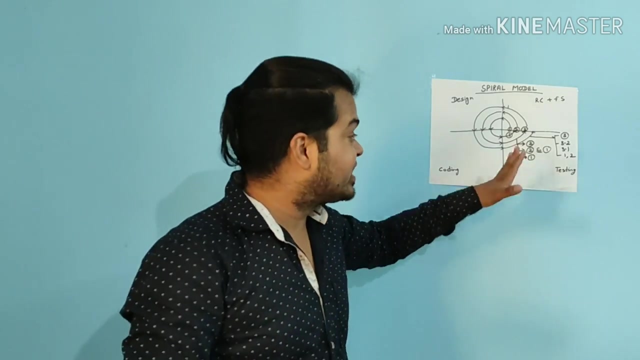 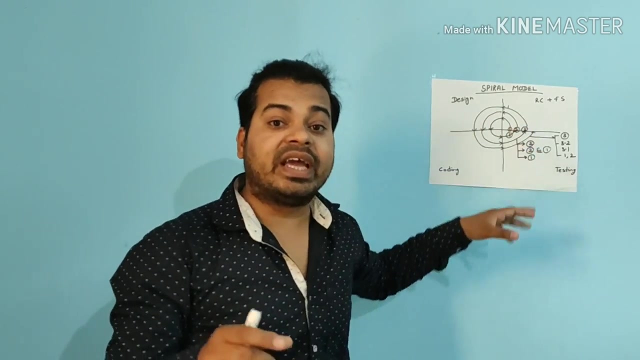 Here requirement changes are allowed Until like what upon model? Here requirement changes are allowed after every cycle. Once first cycle is done, then requirement changes are allowed in the second one. So here the requirement changes are allowed after every cycle. All right, 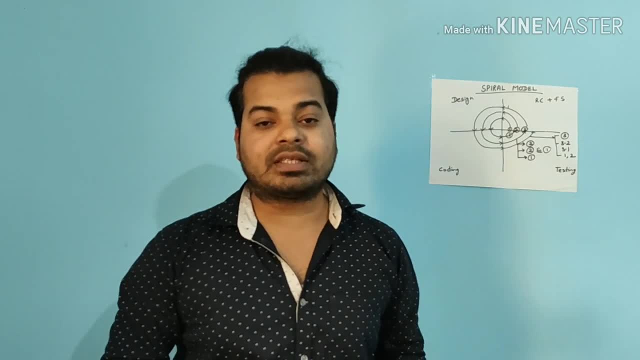 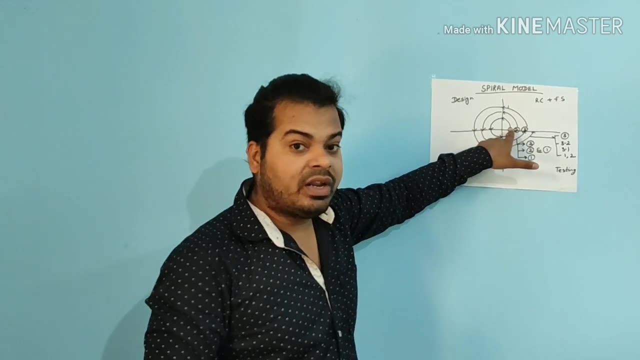 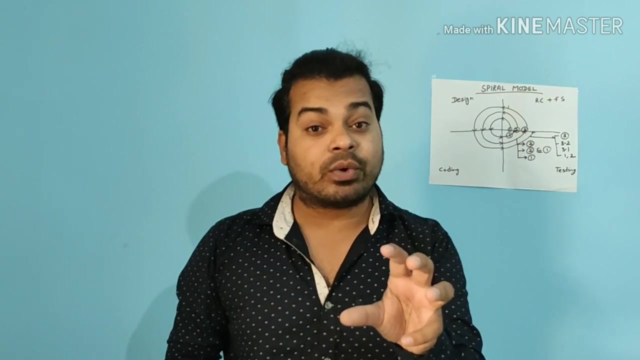 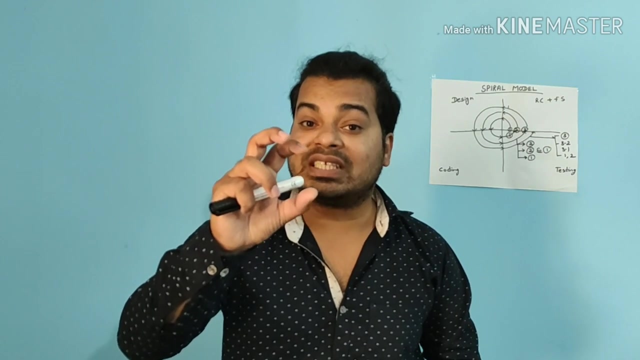 That's it, guys. and second point is: just because we are testing a one module, if it is stable, we are giving to the customer. then only we are picking the second module. it is also called as controlled model. it is also called as controlled model because until unless my first module is ready, it is tested. perfectly fine, it is stable. we. 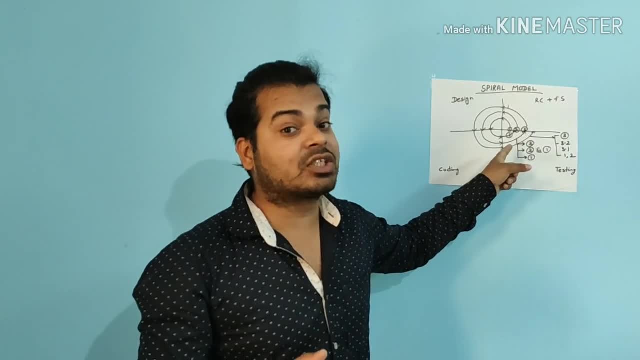 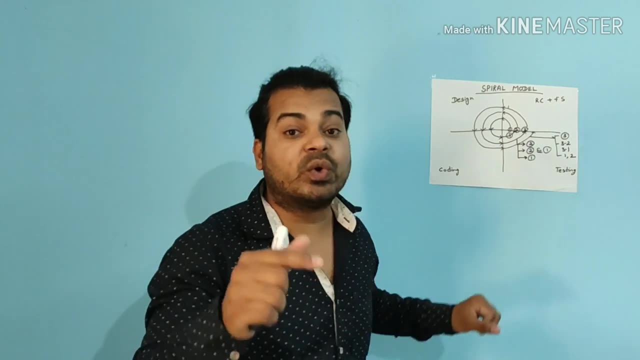 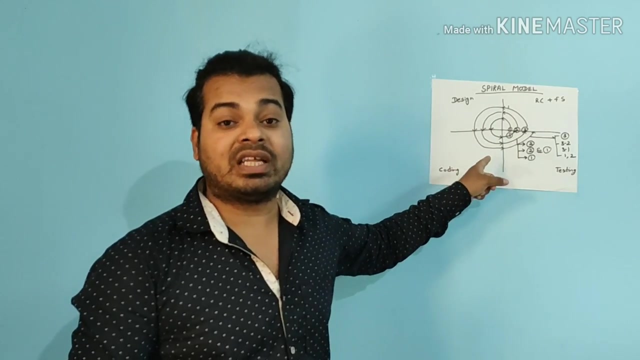 are not going to take the second module. that is the reason it is called as stable module create. here we perform testing in each cycle before going to the next cycle. that is the reason it is. this is the advantages of spiral model, choosing spiral model as a software development life cycle. now the question. 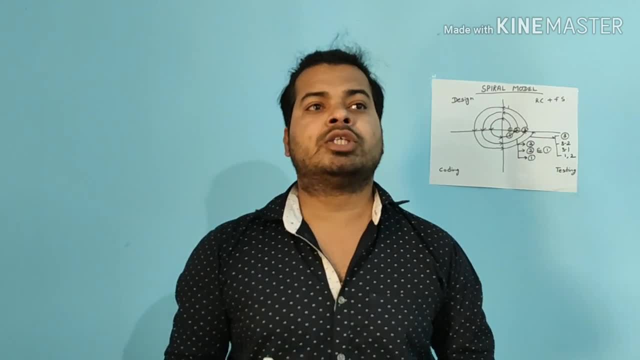 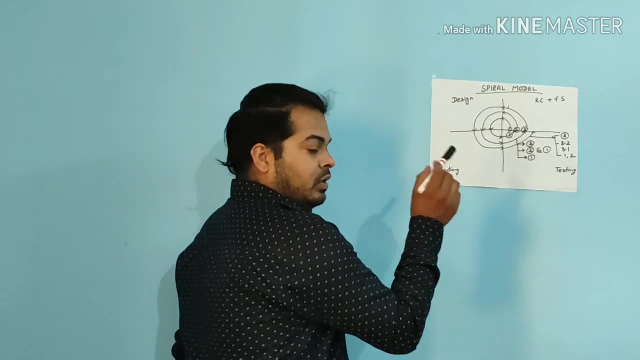 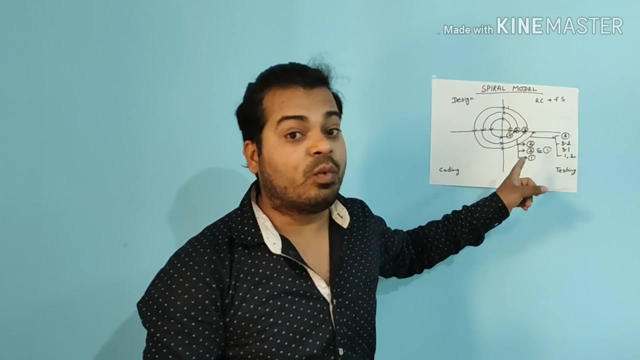 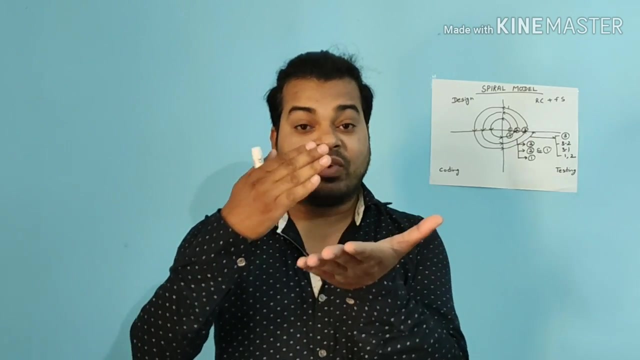 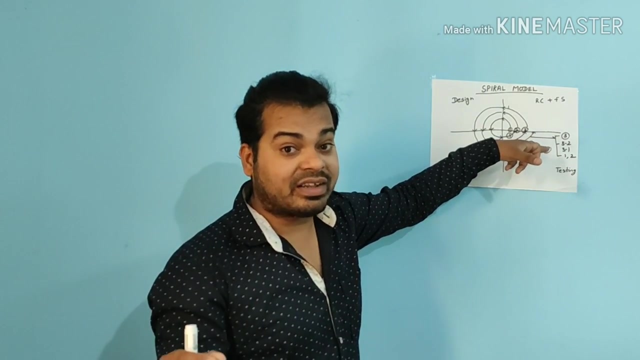 arises. what are the disadvantages of spiral model? so the biggest disadvantages of spiral model is: listen carefully. every cycle of spiral model looks like a waterfall model. if you guys remember what do you mean by waterfall model? once after requirement feasibility study is done, you cannot go back and change the requirement correct. 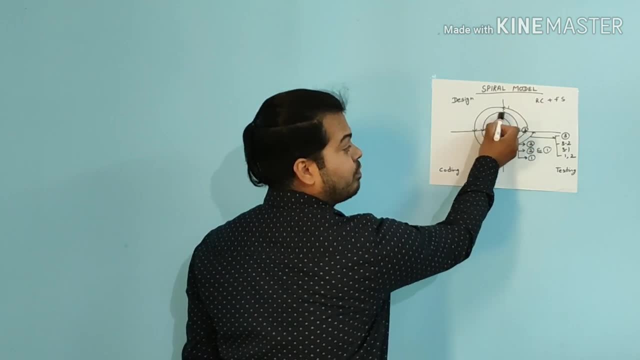 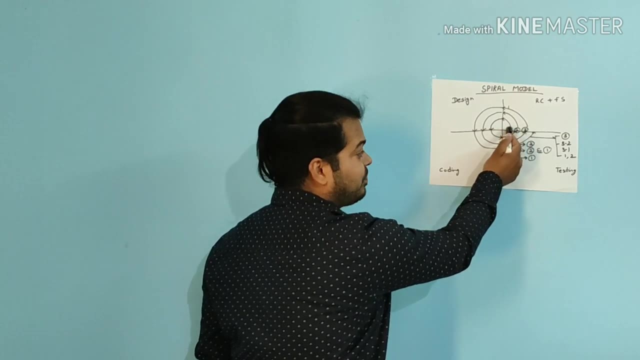 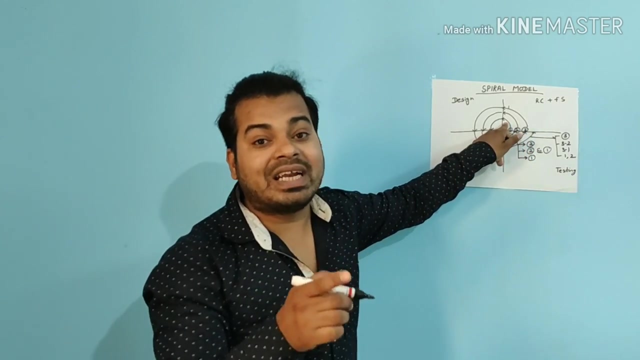 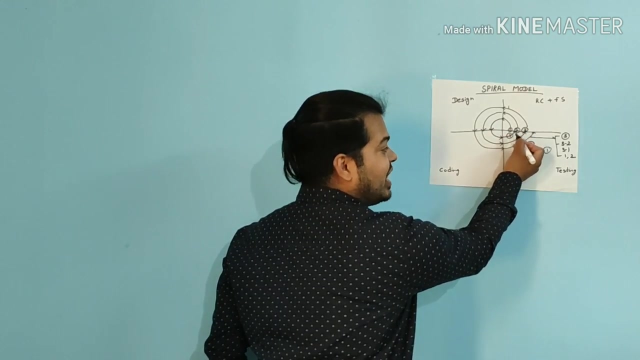 similarly, every cycle of spiral model looks like a waterfall model. so the therefore model. that is when the module first has come and it's requirement collection feasibility study. that it's done, then you cannot go back and change the requirement. requirement is accepted only when my first cycle is tested and